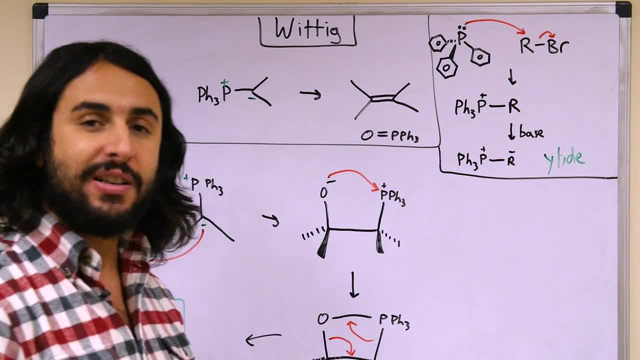 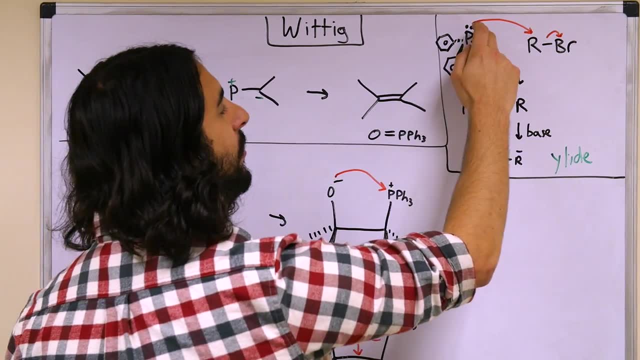 the three benzene rings there and then a lone pair. right phosphorus has five valence electrons, so it can have three covalent bonds and then a lone pair. and then this triphenylphosphine can just do a regular SN2, an alkyl bromide, let's see. 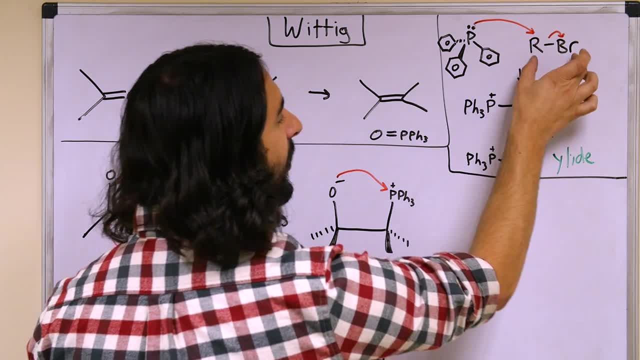 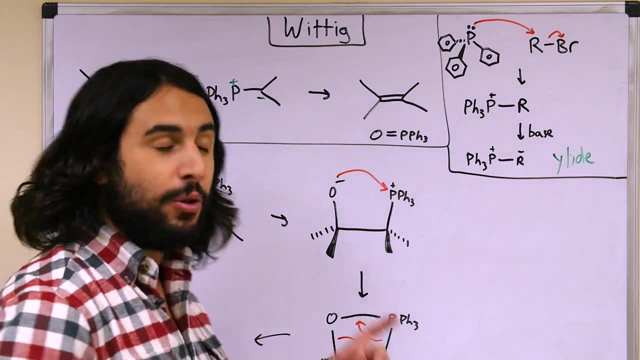 let's say: and so the lone pair is gonna go attack that carbon. this is, there's a polarity to that bond and just regular SN2. so now we will have a phosphorous-carbon bond and furthermore, the phosphorus will have a formal positive charge because it is given one of it's electrons and that lone. 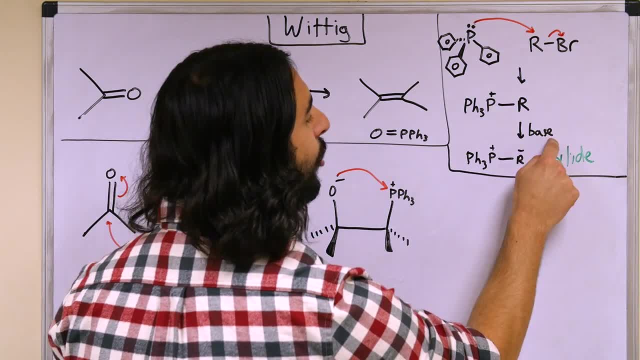 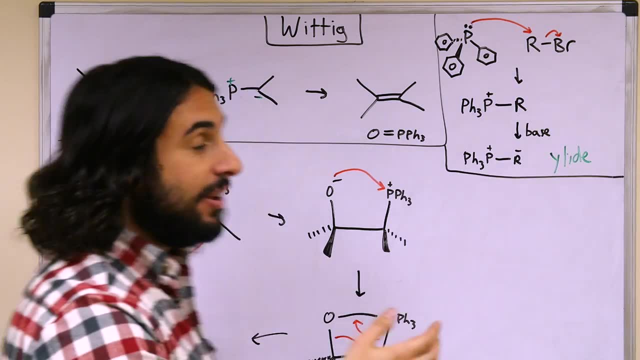 pair to the carbon atom. so now we have that bond and then a little bit of base can extract the proton from whatever. there could be a hydrogen attached here. so R is general alkyl, it could be isopropyl, anything like that. so a base would extract a proton and now we have a. 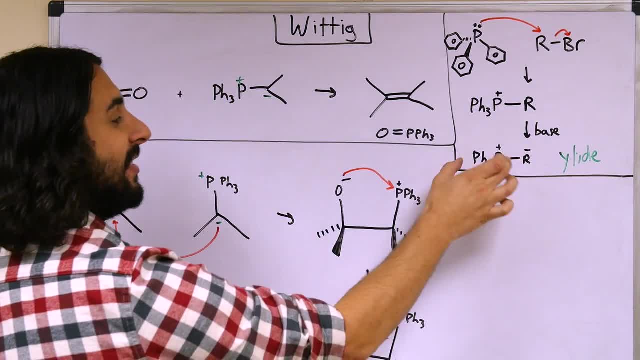 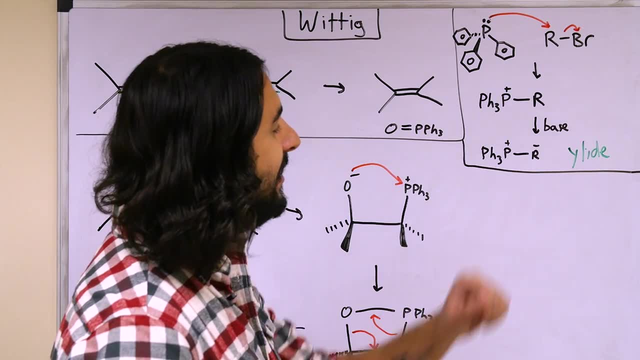 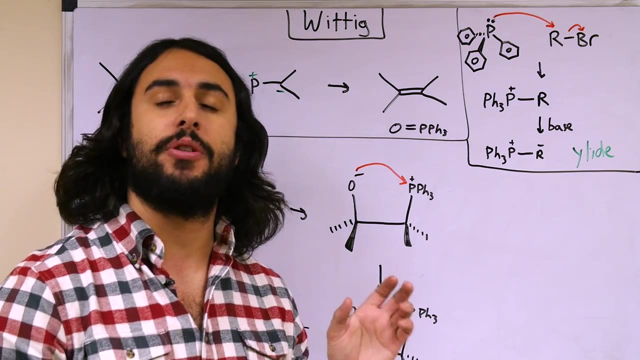 formal negative charge on this carbon. so this, the Wittig reagent, is what results, is an example of a ylid. so a ylid y-l-i-d-e, a ylid is a kind of zwitterion. so we know that a zwitterion is a molecule that has both a positive and 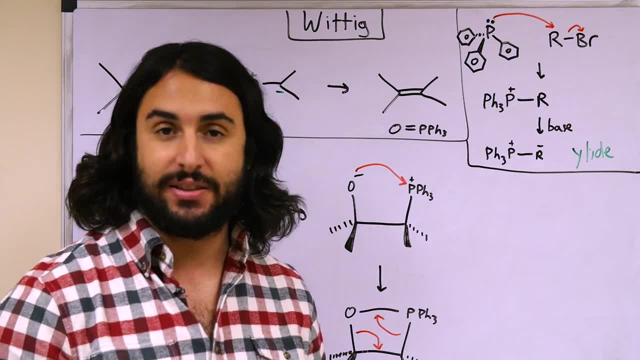 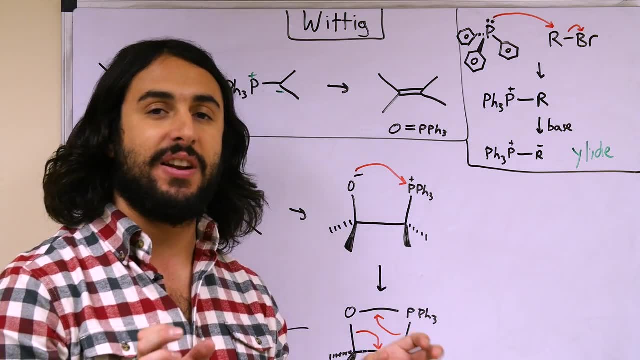 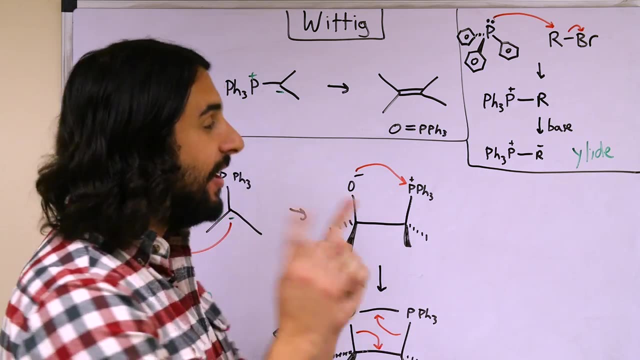 negative formal charge on the same molecule, like an amino acid would be an example. but a ylid is specifically a zwitterion that bears those formal positive and negative charges on adjacent hetero atoms, so hetero atoms being atoms of different elements and then adjacent because they're next to. 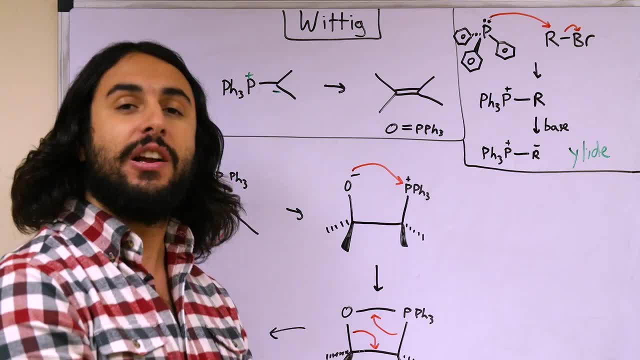 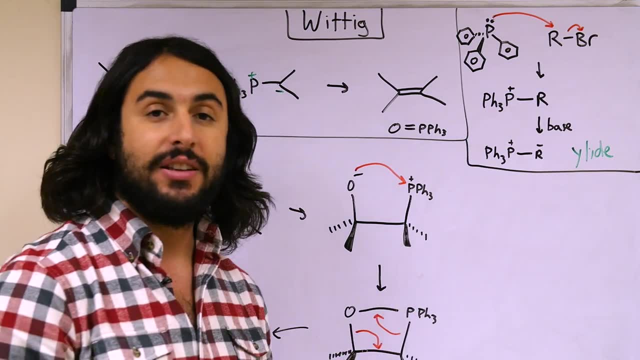 each other. so here is a phosphorus and here is a carbon. they are adjacent. they are different elements, so that qualifies this Wittig reagent as a ylid, and this Wittig reagent is going to react with some carbonyl containing compound. so let's take a look at what this mechanism. 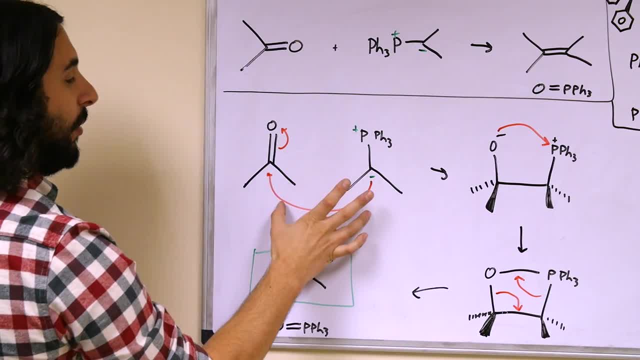 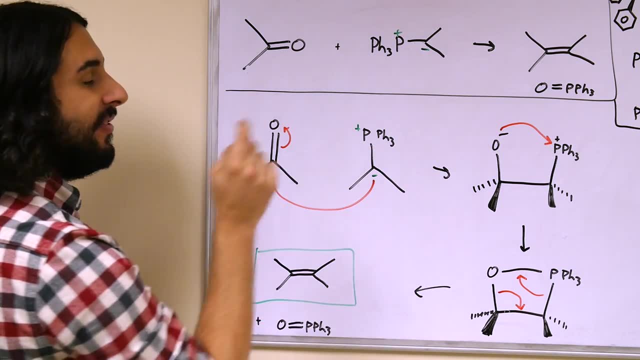 looks like. so I've just taken what's up here and redrawn it to show you what's going on. and we know that the carbon connected to the phosphorous in the Wittig reagent is going to have a formal negative charge, and so, just like with, 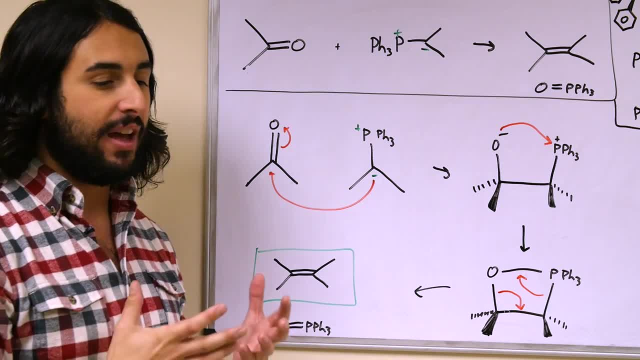 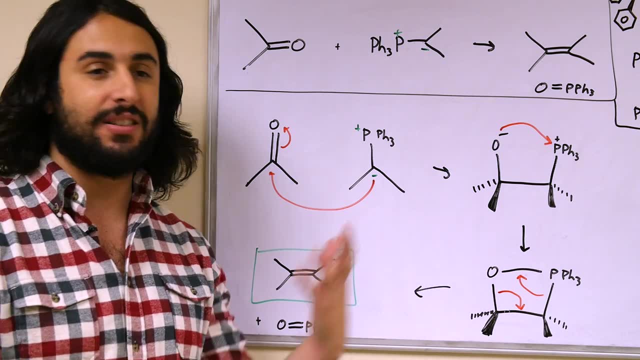 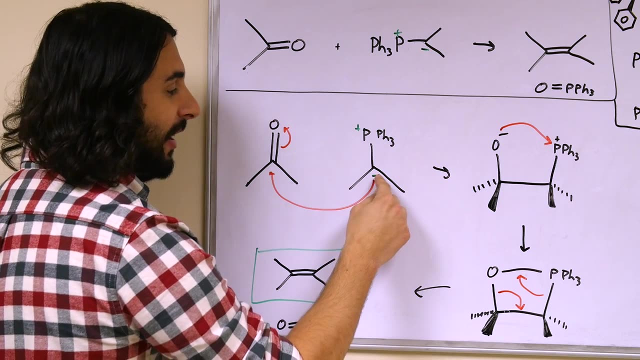 all the other reactions we've been looking at throughout this entire series. we know that reactions are simply examples of electron excess interacting with electron deficiency. so some negativity, some positivity. they react right. so it shouldn't be much of a surprise that a formally negatively charged carbon atom will attack a partially positive carbon. 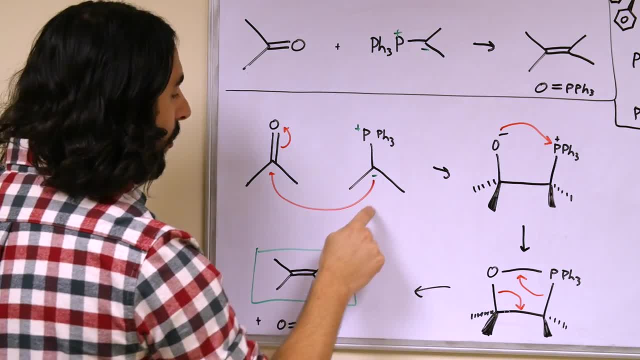 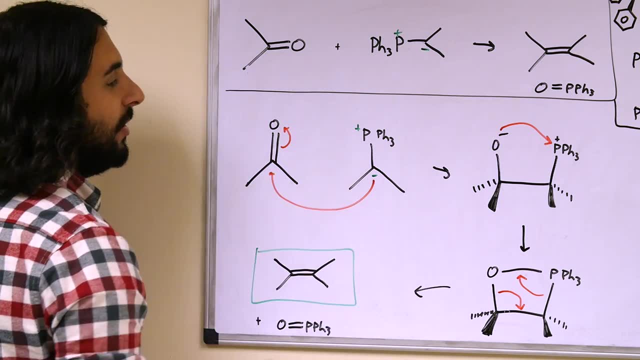 atom in this carbonyl right because of the dipole in the carbonyl. so that will attack here and then this pi bond will go up there. the only way this carbon atom can accept a new bond is by losing another one to go up there, and so these 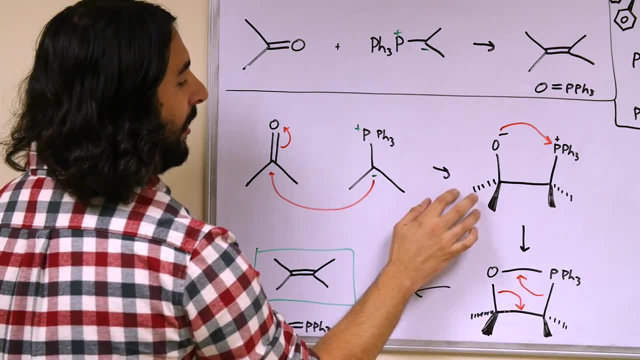 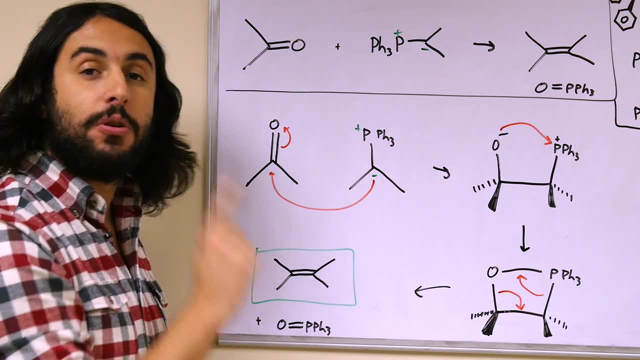 two methyl groups are here. these two methyl groups are here, and now there is a new bond between these carbons. so there, that is there. that's that's one of the two new carbon-carbon bonds that are being attacked by this carbon atom and being formed by the video reaction. so there is that, and now we have this. 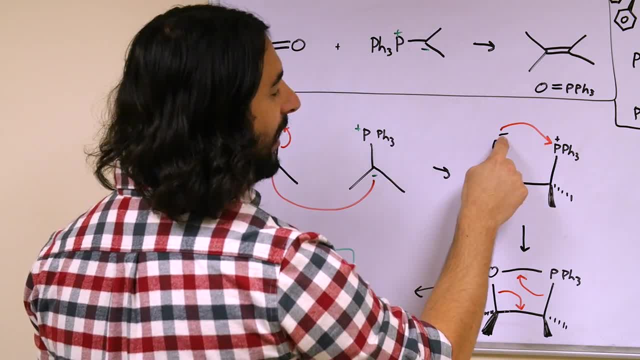 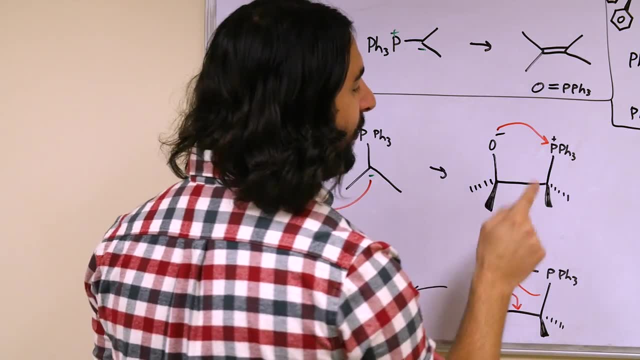 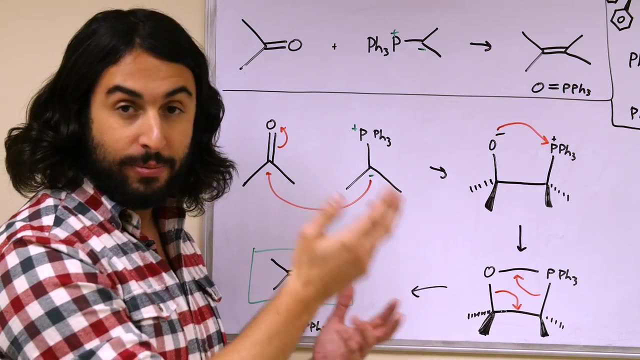 intermediate, and it shouldn't be too surprising, once again, that a negatively charged oxygen would interact with the formally charged phosphorus in an intra-molecular fashion. so phosphorus can accommodate five bonds. that violates the octet rule, as can almost any atom, apart from oxygen, carbon nitrogen, these, 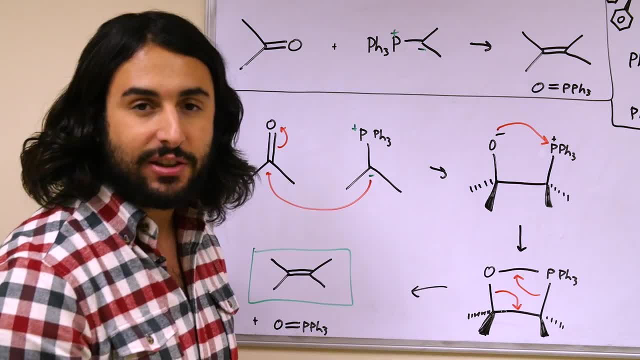 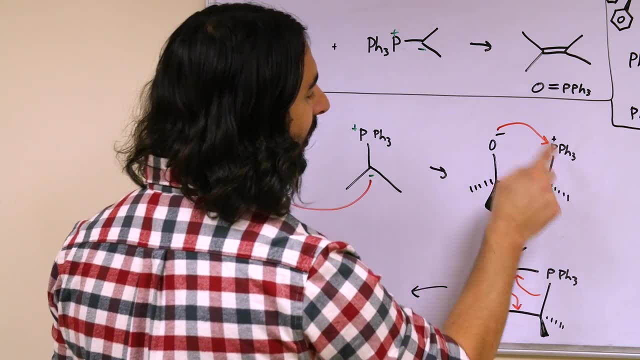 ones. so once we're down a row, phosphorus, five valence electrons, 5 covalent bonds works perfectly fine. so phosphorus will be bound to theediac and it should not be too late to be found in the ground later on. those three phenyl groups, this carbon down here, and now a new bond to this. 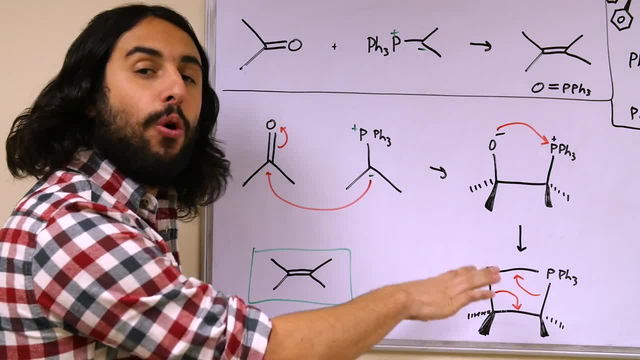 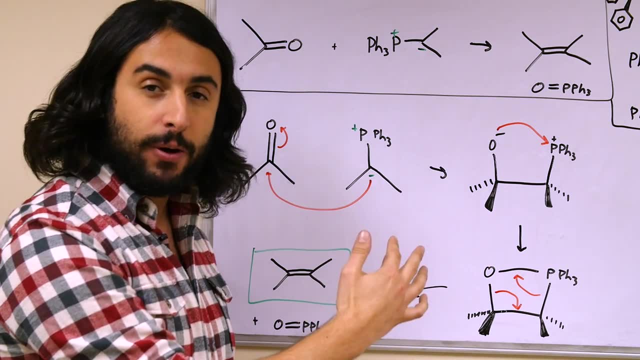 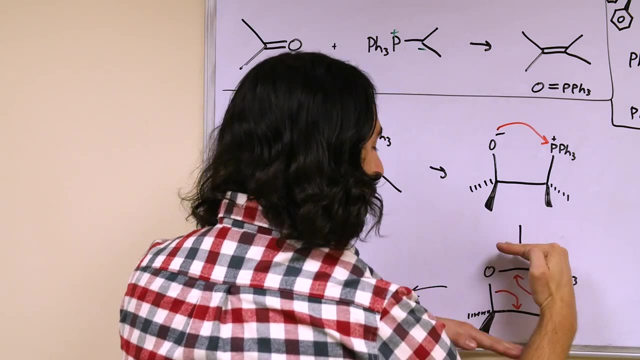 oxygen. so here we have this new cyclic, this four-membered ring intermediate, and this is where something very interesting can happen. the bonds can rearrange to go back to the way they were, or they can cyclize in a different way and go like this, where we're basically gonna gonna flip these bonds. 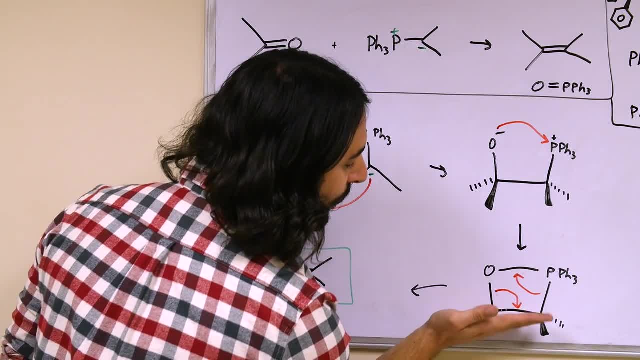 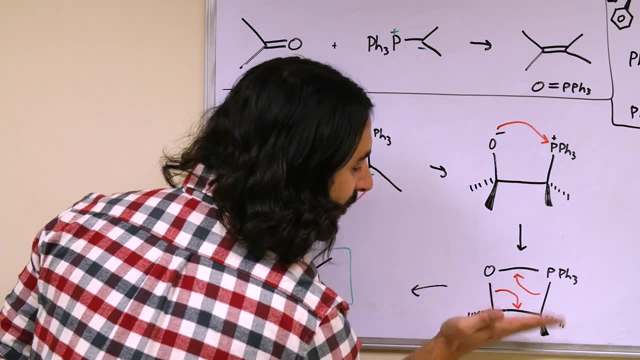 in such a way so as to have this bond go and form a pi bond here between the two carbon atoms that had the new sigma bond in the first place. so that will snap shut there, forming the alkene product, and then this one can flip up this way: 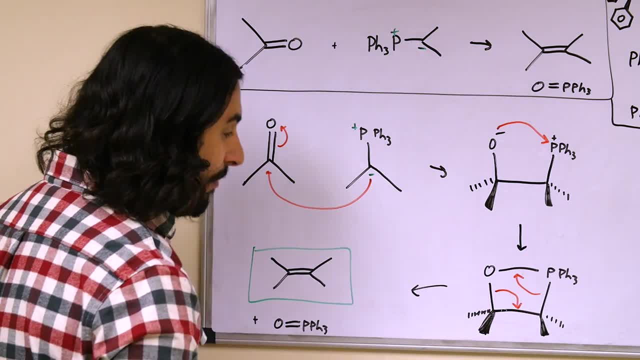 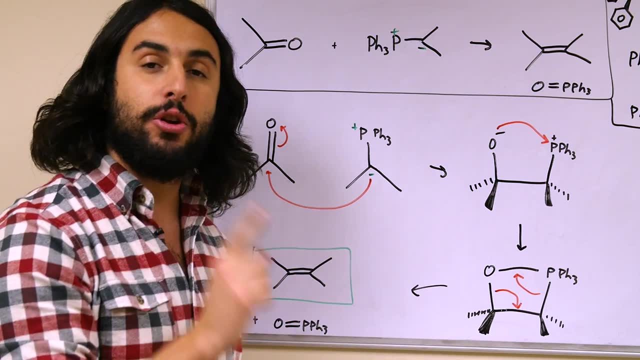 to form a double bond between phosphorus and oxygen to generate the byproduct. so that's sort of the key step in giving us our alkene product. so both of the new bonds, the sigma and the pi bond, are being formed between these two carbons. 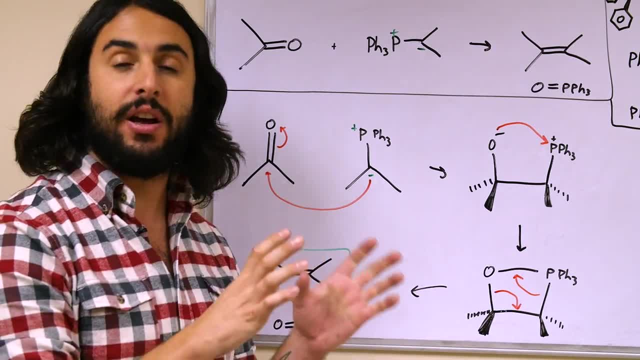 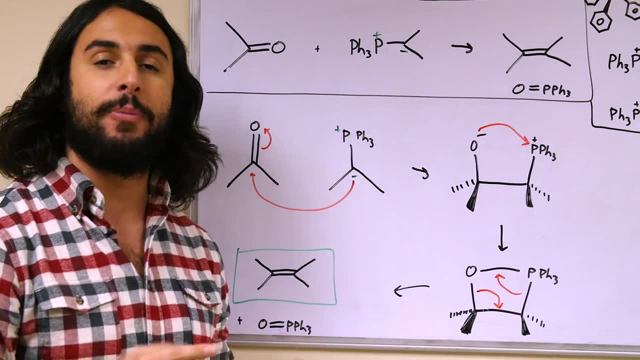 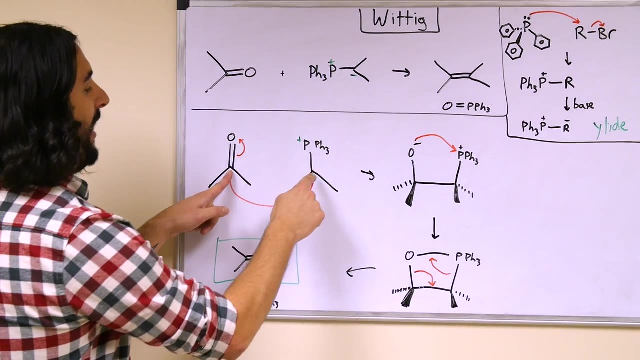 so when you look at a Wittig reaction and are looking at the substrate and the Wittig reagent, what we want to understand is that we are always forming two new carbon-carbon bonds and both of them are occurring between the carbonyl carbon and the negatively charged carbon.